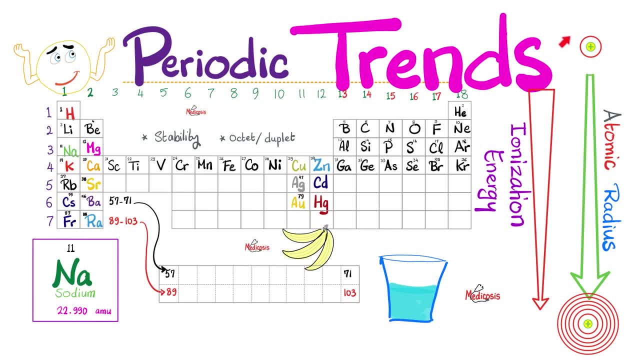 radius keeps getting bigger and bigger and bigger. You go from this to this, because this one had only one shell, But look, here we have seven electron shells. So the trend is that the atomic radius increases down a group. And since it's a trend in the periodic table, 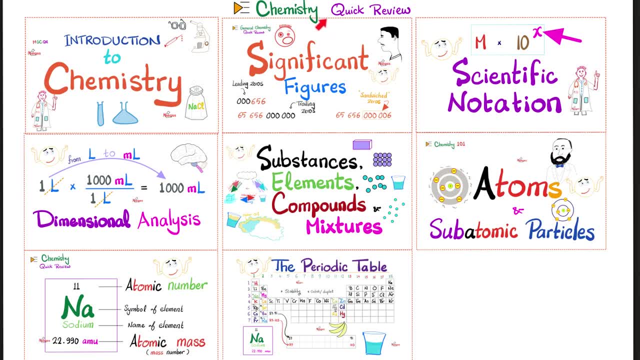 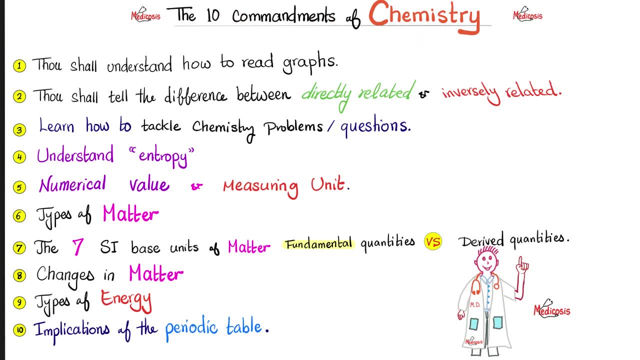 it's called periodic trend. Please watch the videos in this chemistry quick review playlist. in order, Hit the like button. If you remember my 10 commandments of chemistry, many of them included matter and energy, as well as the implications of the periodic table Matter. 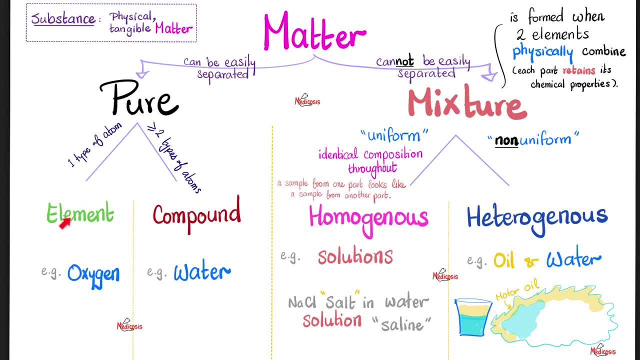 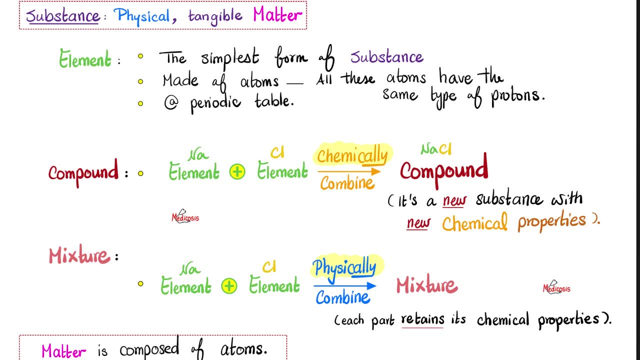 could be pure or could be a mixture. Pure matter could be an element or a compound. Today we're talking about the trends of the periodic table of the elements. What's an element? It's the simplest form of a substance, which is physical matter. An element is made. 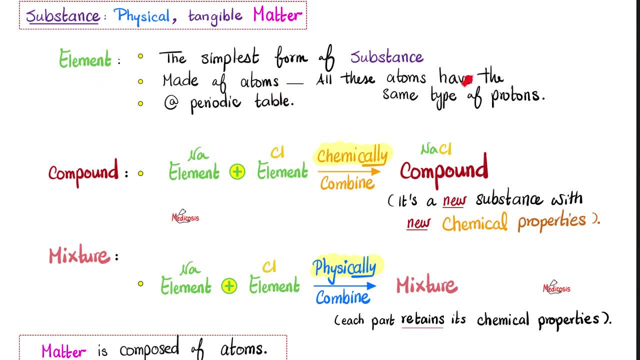 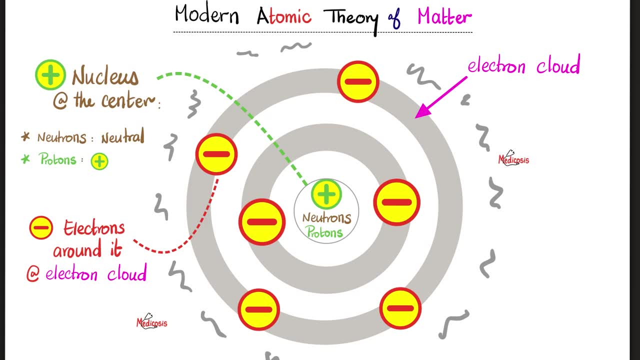 of atoms, For example oxygen. An element is made of oxygen atoms. Here is a very simplistic view of the atom. In the center we have the nucleus. Around the nucleus we have shells that contain electrons. Are these shells well demarcated, like drawn with a pencil? No, they are very vague- poorly. 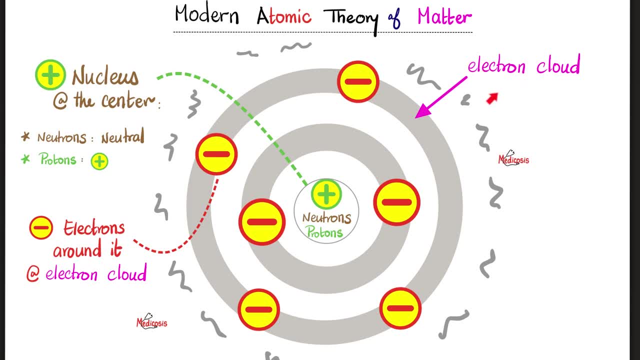 demarcated. You can call them an electron cloud: Hazy, blurry, vague, unclear. The nucleus is positive. Why? Because it has neutrons which have no charge, and protons, which are neutrons which have positive charge. So overall, the nucleus is positive And around. 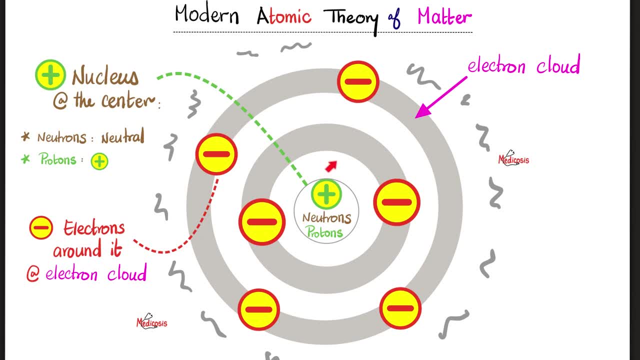 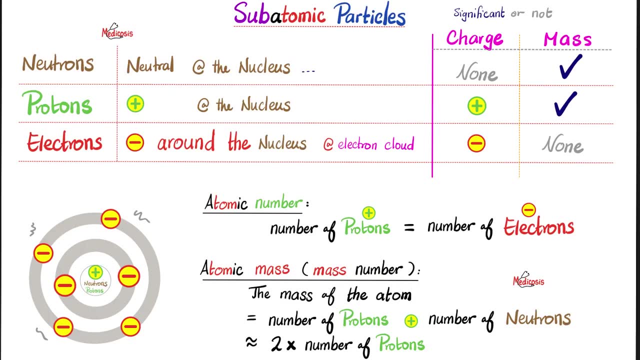 it. we have a nucleus which is negative. The positive and the negative cancel each other out and you end up with a neutral atom. Neutrons are neutral and located in the nucleus. Protons are positive, also in the nucleus. Electrons are negative around the nucleus, The neutrons. 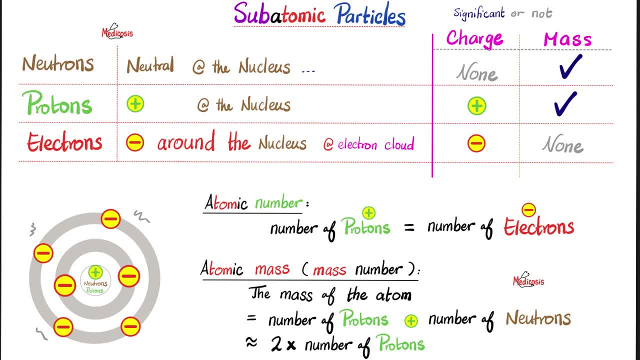 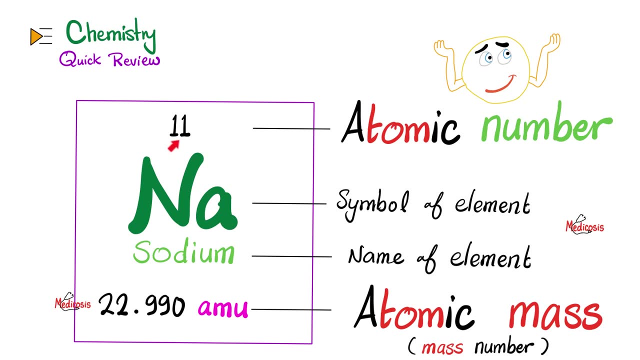 are neutral. Protons are positive, Protons are positive, Electrons are negative. Let's talk about the masses. This is so tiny, it's almost insignificant, You can ignore it. Here is the atomic mass and here is the atomic number. The atomic number is the number of protons. It's also 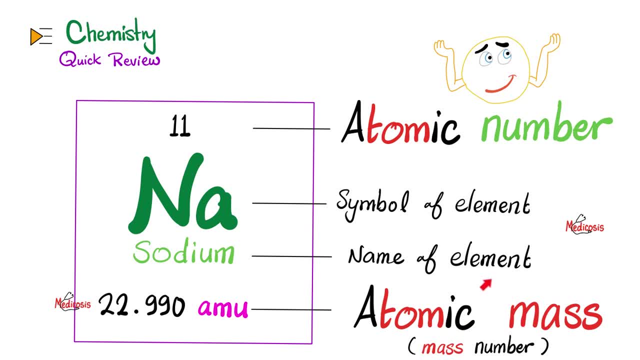 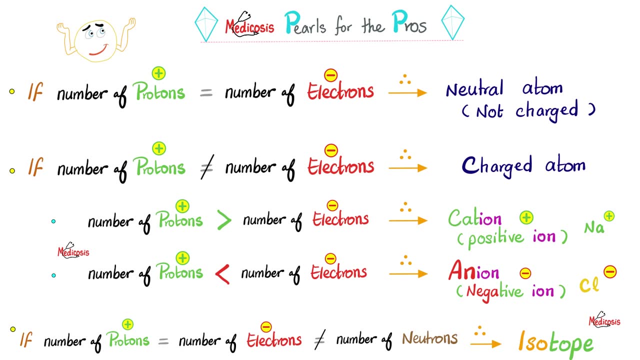 the number of electrons. The atomic mass or the mass number, roughly speaking, is the number of protons plus the number of neutrons. Why isn't it a whole number? Because it's a weighted average, as we have discussed before. Number of protons equal the number of electrons. 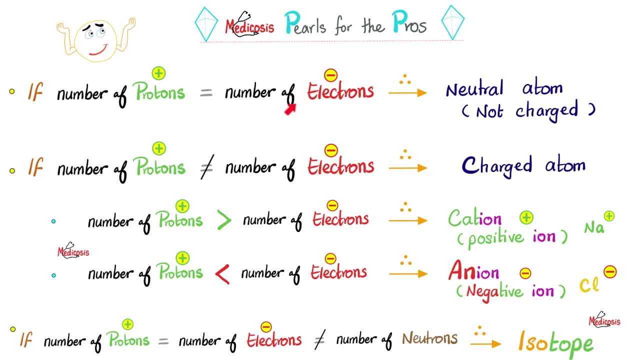 this is called the atomic number. Since the positive charges equal the negative charges, you have a neutral atom. but what if the number of protons exceed the number of electrons? then you have a positive ion. What if the number of the negative electrons exceed the? 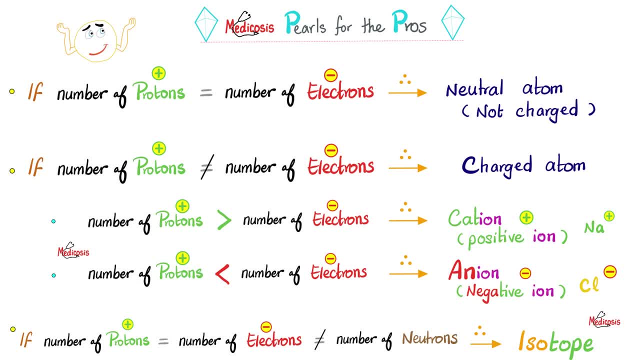 number of positive protons, then you have a negative ion. What if the number of protons equal the number of electrons, but the number of neutrons is different? that's an isotope, such as carbon 13,, carbon 14, etc. 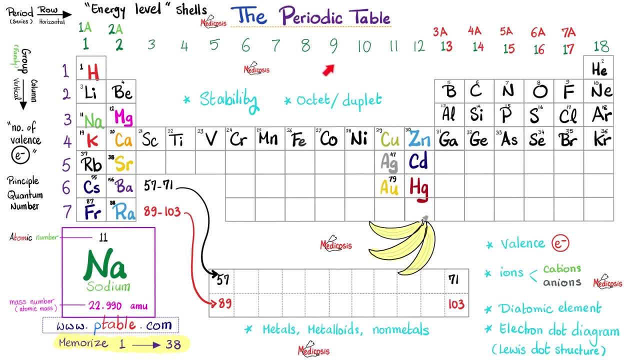 '' about the periodic table. Don't forget, we go horizontally. We call them periods or rows, or a series of elements. Number one has one energy shell. How about period number two? Well, each element has two shells of electrons. In period three, you have three shells of electrons. I said 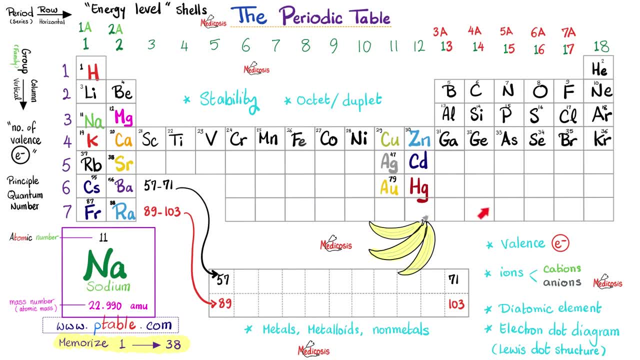 shell, not subshell. How about period number seven? It has seven shells of electrons. Next let's go vertically. Now we call this a group or a family of element. Group one has one electron in the outermost shell, called the valence shell. Group two has two electrons. Group 3a or 13, three electrons. 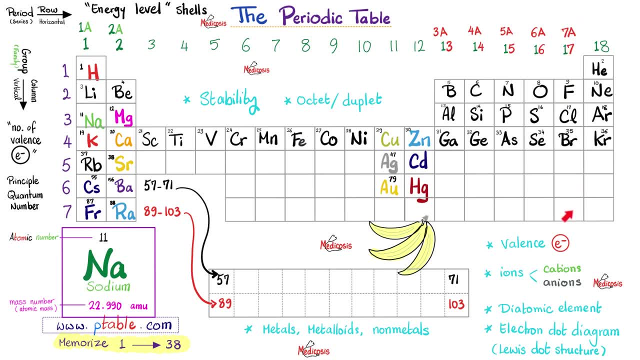 Group 17 or 7a: seven electrons in the outermost shell. Group 18, the noble gases: eight electron in the outermost shell. If you have eight electrons in your outermost shell, you are called subshell Stable, And this is the octet rule. Octet means eight. Now let's talk about the periodic trends. 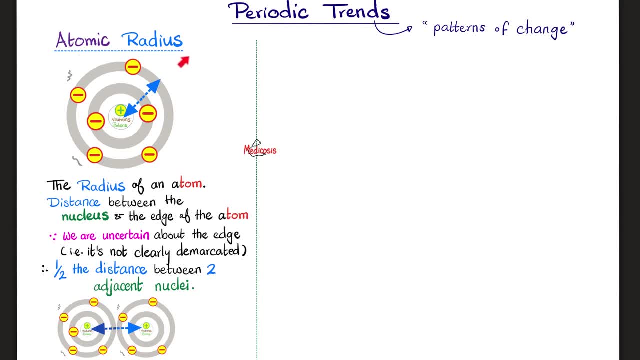 First atomic radius Definition. atomic radius, the radius of the atom. Thank you, Captain Genius. And of course the radius is half the diameter. So the radius is from the center to the outermost part, ie it's the distance between the nucleus of the atom and the edge of the atom Is the edge. 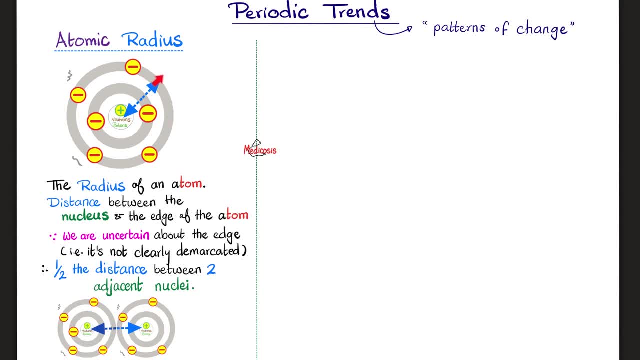 of the atom, clearly demarcated, As if it was drawn by a shot. Is it a sharp pencil? Heck? no, It is vague. We're uncertain about the edge of the atom. It is not clearly demarcated. Therefore, there is a better definition. Here's an atom. Here's another atom. 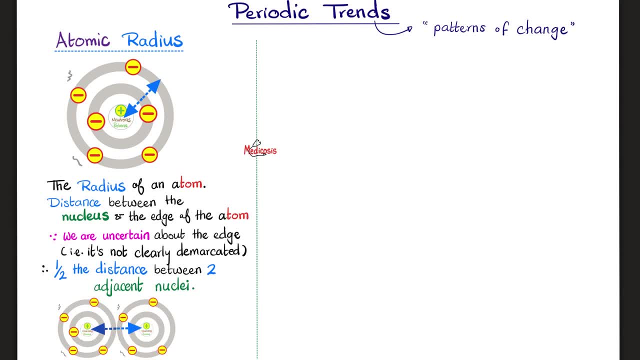 Take the distance between this nucleus and this nucleus and give me half of that distance, and that will be the radius of the atom. This definition is more accurate than this definition. Let's talk about the atomic radius trend down a group and across a period. 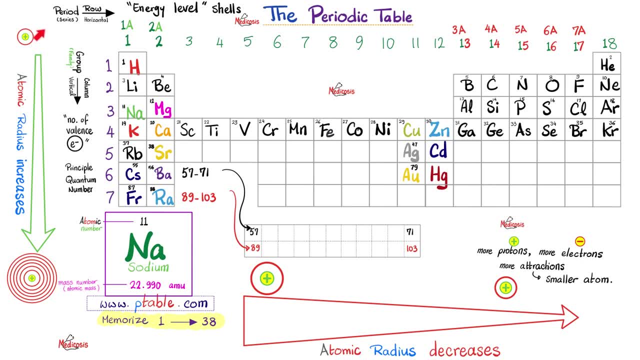 First down a group. Think about it. We went from one electron shell into seven electron shell, So of course this atom is way bigger than this atom. The atomic radius here is bigger than the atomic radius here. Makes perfect sense. So as I go down a group, my atomic radius keeps getting. 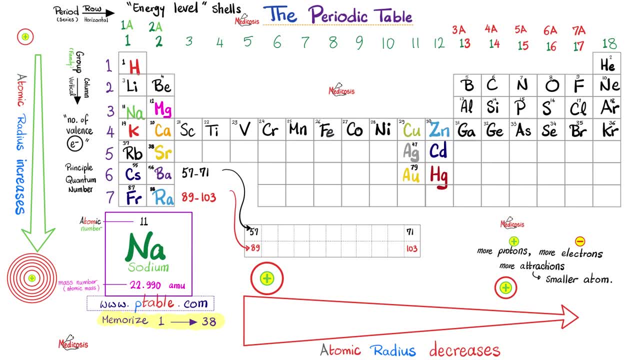 bigger and bigger and bigger. We're done with down a group. Now let's talk about the atomic radius trend across a period. As I go from here to here, what do you think is going to happen? Well, let's see. I went from three protons and 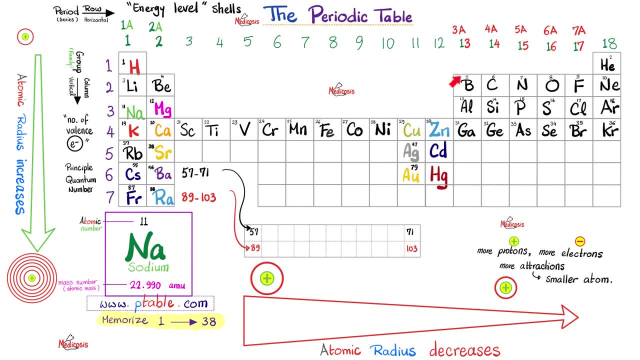 three electrons to four protons, four electrons, five protons, five electrons, six protons, et cetera, et cetera. So, as I go from the left to the right, the number of positive protons go up and the number of negative electrons go up, And, as you know, opposites attract. 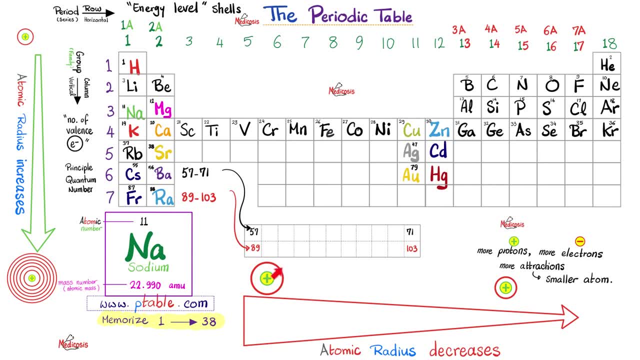 which means on the left, the attraction between the positive and the negative is weak. But as you go to the right- because you're adding more protons and more electrons, you're adding more positive charges and more negative charges- you're adding more attraction. 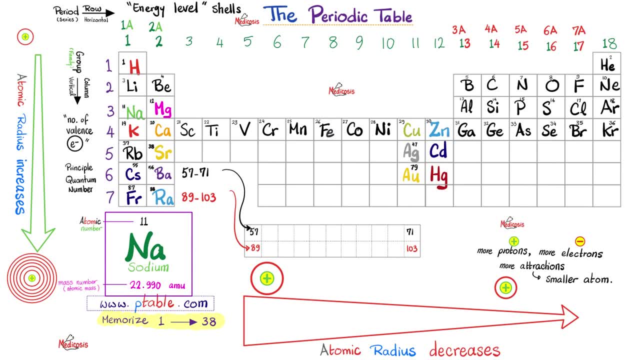 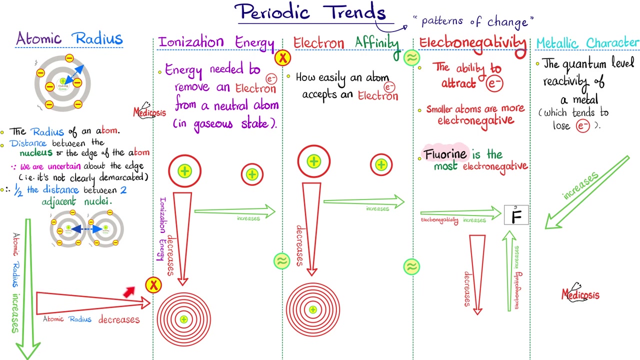 forces, which means the atom will get smaller and smaller and smaller because the positive nucleus is attracting the negative electrons more and more and more. So you shrink and shrink and shrink. So as you go across a period the atomic radius decreases. So atomic radius down a group, it goes up across a period, it goes down. Next, ionization. 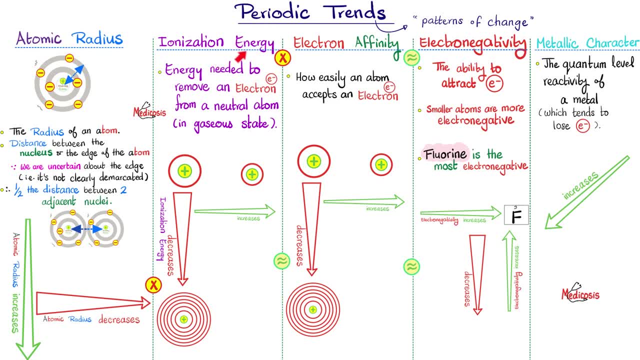 energy. What the flip is that. Think about it. It's called energy ionization. What's an ion? Oh, an ion is something that's not neutral. Exactly Here we're trying to remove a negative electron. When you remove a negative electron, the atom becomes a positive ion, ie a cation. 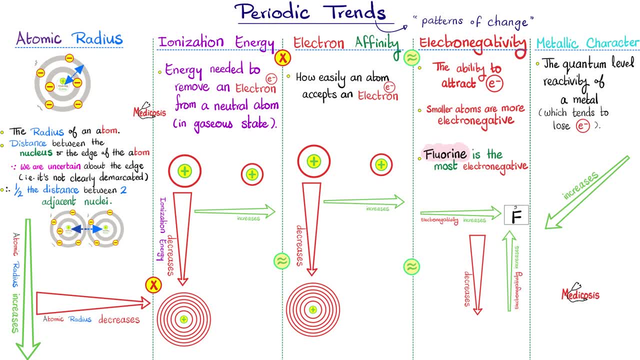 So think of ionization energy as a positive ion. So think of ionization energy as a positive ion, as the energy needed to make a positive ion. It's the energy needed to remove an electron from a neutral atom in the gaseous state. Now let's think about the trend. Let's start on the upper left. 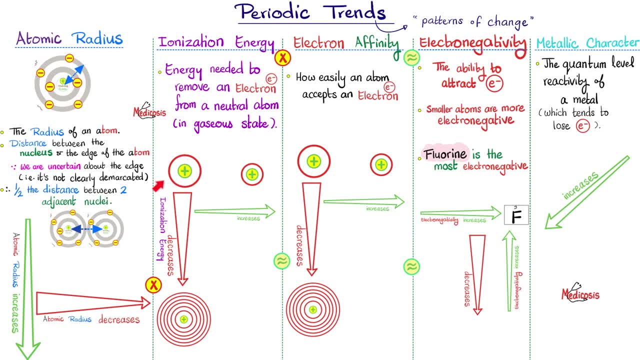 part of the periodic table. The atom is small, which means the outermost electron is close to the nucleus, Yes, which means the positive charge and the negative charge are attracting each other, which means it's very difficult. It's very difficult to get that electron out of the atom because it's close enough to the positive. 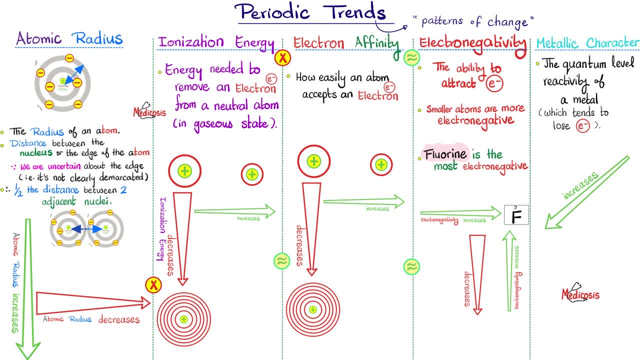 nucleus. Conversely, as you go down, down, down, down, down down a group- look what happened here- The furthermost electron is here, which is far away from the positive nucleus, which means it's easier to remove that electron compared to that electron, ie by going down a group. 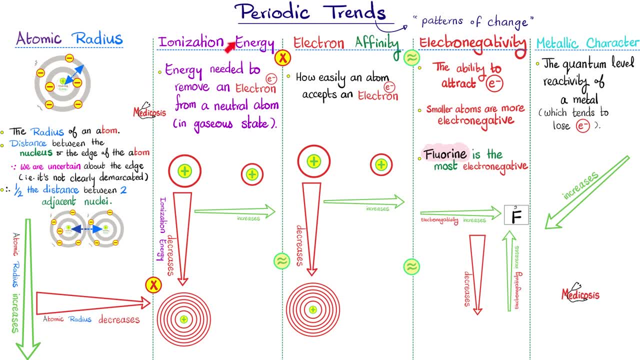 your ionization energy decreases. The energy needed to remove an electron gets lower and lower and lower. because it gets easier to remove an electron the farther it gets from the nucleus, And that was the trend of ionization energy down a group. How about across a period? Think about it. Across a period, the electron 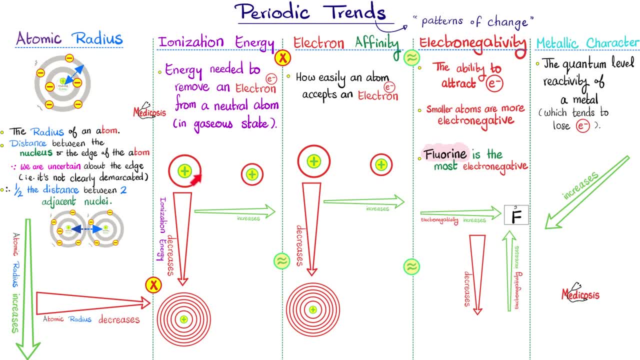 keeps getting closer and closer and closer and closer to the nucleus, which means it gets harder to remove that electron from the atom, ie it takes more energy from the nucleus, which means it gets energy, which means ionization. energy goes up Next. electron affinity has the opposite definition. 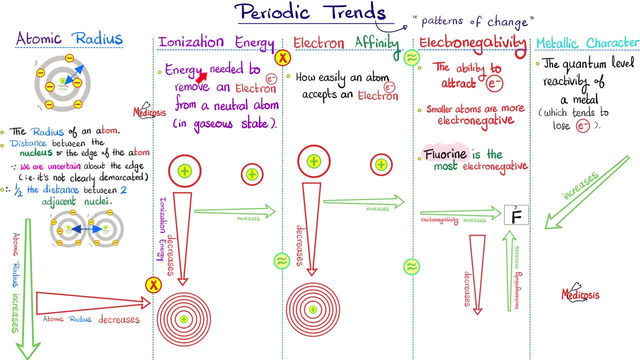 of ionization energy. Ionization energy was trying to remove an electron away from the atom. But look here at electron affinity. This is how easily an atom attracts and accepts an electron. Go away versus come closer. So the definition is the opposite. However, the trend is the same: Down a. 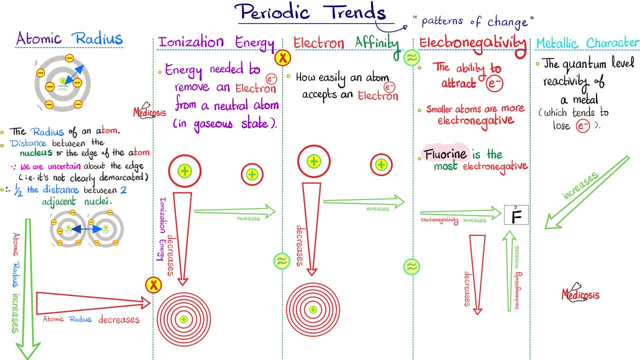 group. electron affinity decreases Across a period. it increases, just like ionization energy. But I don't get it. Let's think about it. Affinity means love. Which two people love one another the most? Those who are very close to each other. ie a positive nucleus and a negative electron. 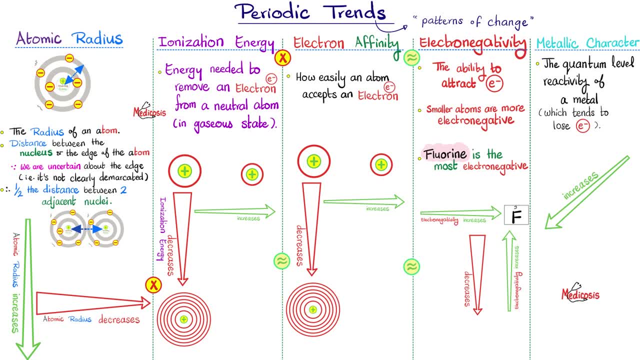 or those who are far away from one another. Of course, these two love each other more Perfect. So the electron affinity here is high. As you go down, electron affinity is high. As you go down, affinity decreases. Oh, that makes sense. Moreover, when you go across a period, 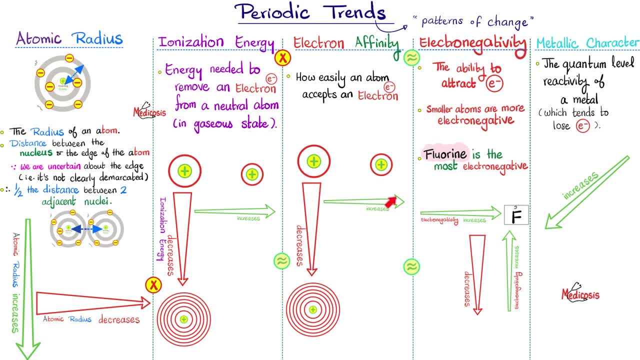 you keep adding more positive charges and more negative charges. so they attract one another more. They tend to love each other more on the right side than on the left side. So across a period, electron affinity increases. The fourth concept is electronegativity, As you know. 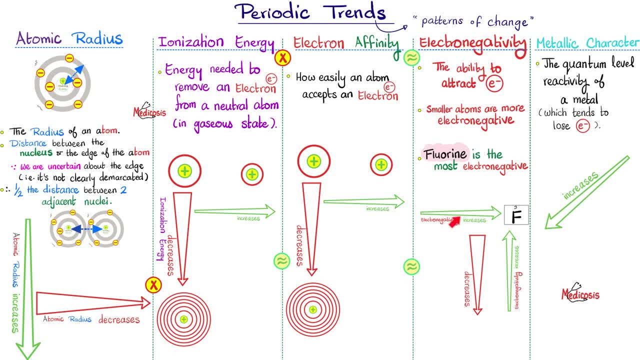 electrons are negative. I want you to look at your periodic table. Let's look at sodium, for example, which is number 11.. I want you also to look at chlorine, which is number 17.. They are in the same row, in the same period, correct? Yes, they are. Which one? 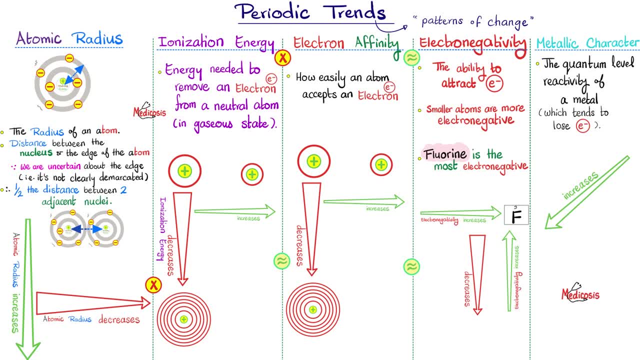 has more positive charges, ie protons. Answer: chlorine. of course the one on the right side, Chlorine, has more protons than sodium. Okay, let's talk about electrons. Which one has more electrons? Is it sodium or chlorine? 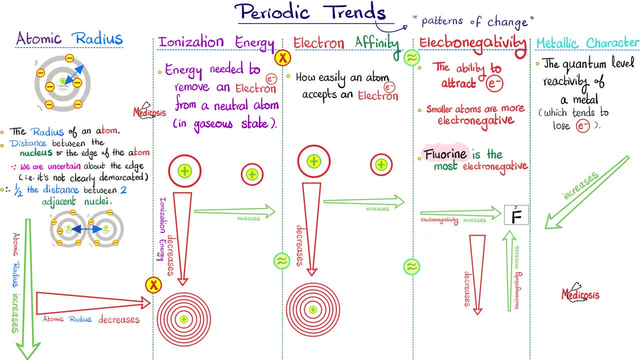 Answer: also chlorine, Nice. How many electrons does sodium have in the outermost shell? The answer is one. I said shell, not subshell. The configuration of sodium is 2, 8, 1.. Two electrons in the first shell, eight in the second shell, one in the third shell. How about chlorine? 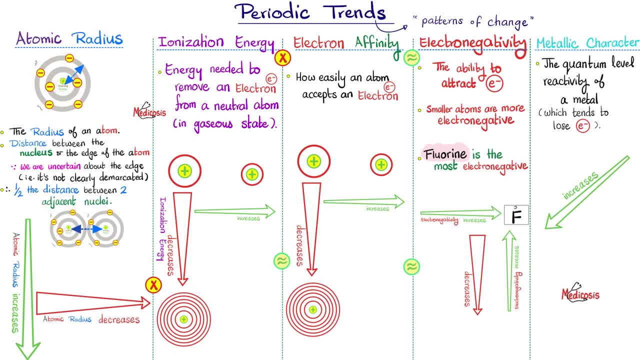 Chlorine has 17,, so the configuration is 2, 8,, 7.. And to achieve stability, ie the octane sodium would love to lose an electron, But chlorine, the one on the right side, would love. 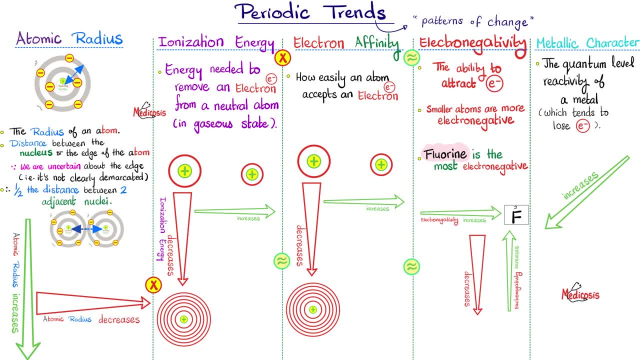 to gain another electron, to become octet, to become like the noble gas argon, which means chlorine has more ability to attract an electron, therefore higher electronegativity. So across a period electronegativity increases. Let me make it easier for you. Who's the most electronegative? 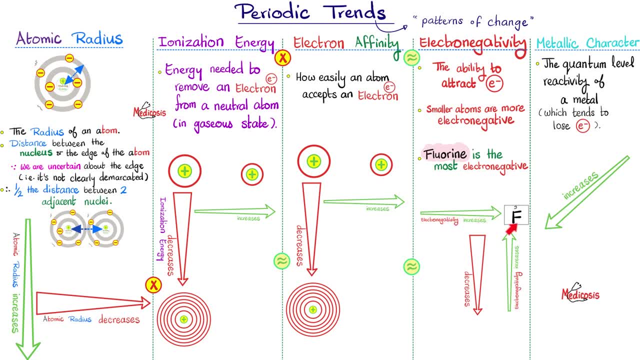 Answer: fluorine. So if you're getting closer to fluorine, electronegativity goes up. Look at this: I'm going to the right, Oh, and fluorine is on the right, Exactly, If you're going towards fluorine, if you're going to the most electronegative, therefore electronegativity. 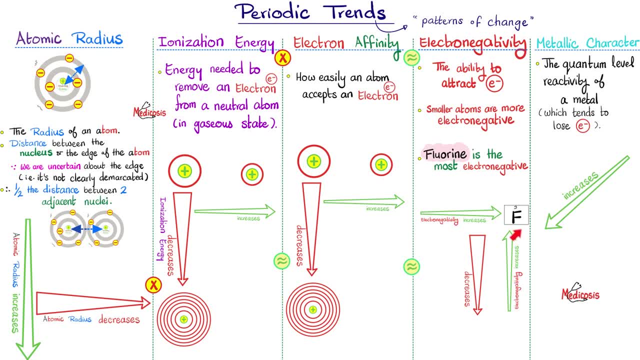 will increase across a period. If you go up a group, you're getting closer to fluorine, so electronegativity increases. But if you're going down a group, away from fluorine, away from the most electronegative, therefore, electronegativity decreases On average. 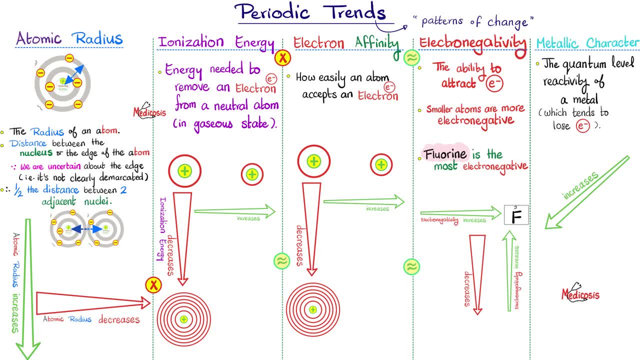 smaller atoms are more electronegative than large atoms, which makes sense, because if you're small, it means there is less electron shielding, ie less electrons are covering around the nucleus, So it is easier for you to attract an electron from the outside world. 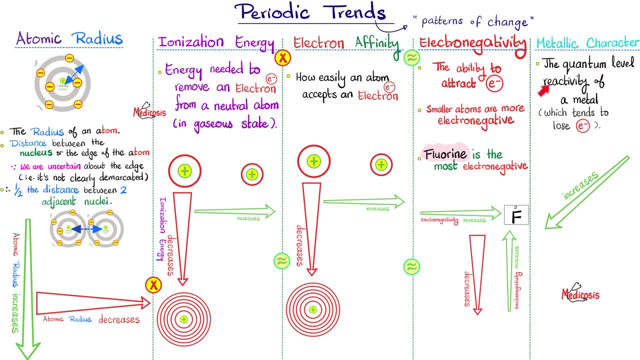 Last metallic character. What's that? It's the quantum level reactivity of a metal And, as you know, reactivity of the metal is based on the tendency to lose electrons, which is the opposite of electronegativity, because electronegativity was about 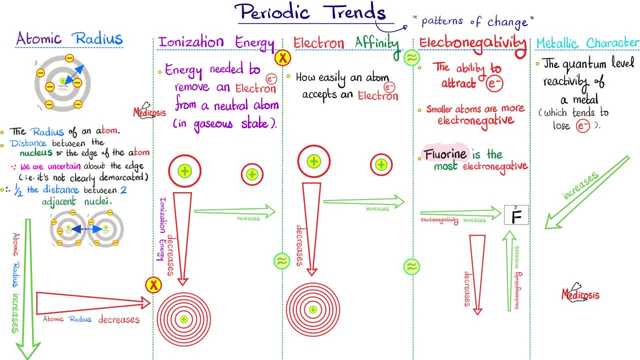 attracting an electron. But metallic character is about losing an electron And since electronegativity went up as I go up and to the right, therefore metallic character has to be the opposite: It increases as I go down and to the left. See, chemistry makes. 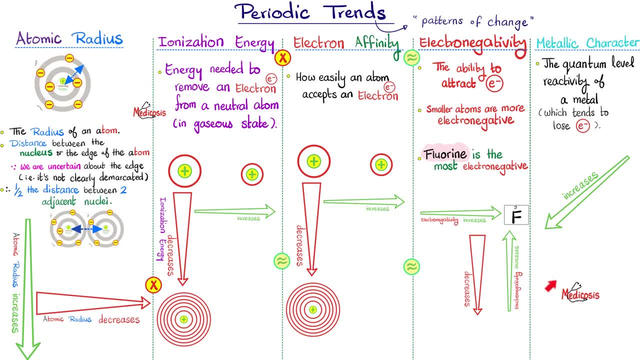 so much sense once you understand what the flip you're talking about. So let's summarize: Atomic radius: Down a group, it increases. Across a period, it decreases. If you want ionization energy, it's the opposite. Down a group, goes down. Across a period, goes up. 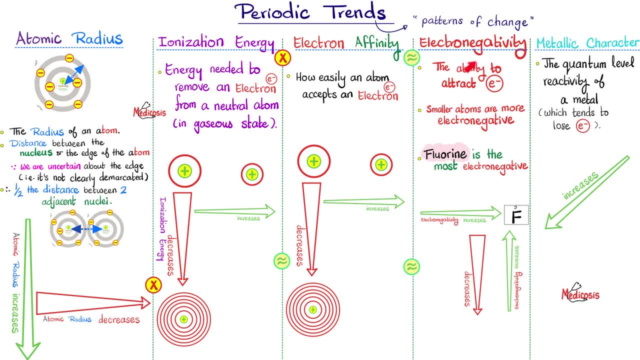 Then electron affinity is the same trend, Electronegativity almost the same trend. Just remember, fluorine is the most electronegative. How about metallic character? The exact opposite of electronegativity. Electronegativity goes up if you go to the right and upwards. 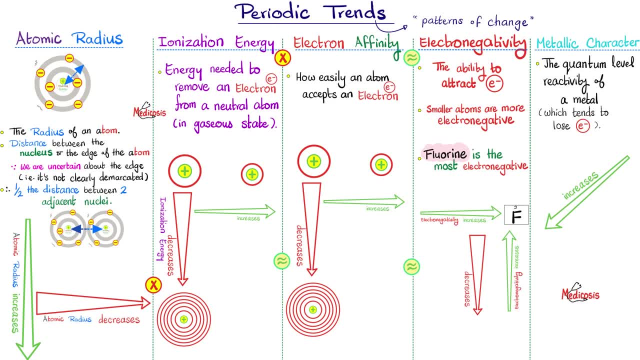 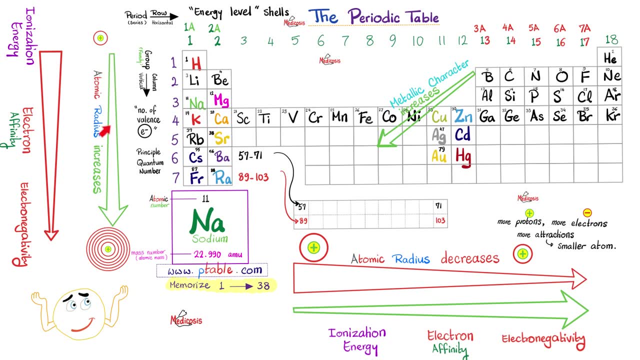 Metallic character goes up if you're going to the left and downwards. So let's draw all of this on the periodic table. First, atomic radius: If you're going downstairs it increases. Conversely, ionization, energy, electron affinity and electronegativity decrease as you go down. 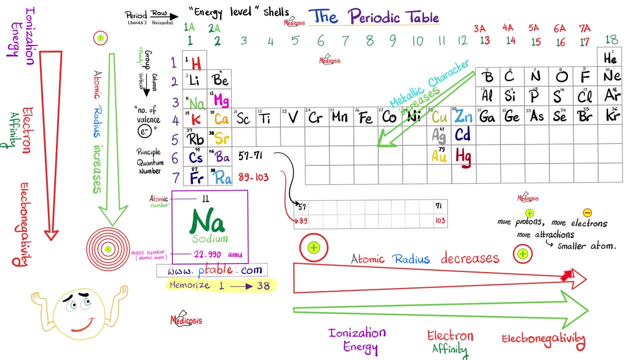 Let's go across a period. Atomic radius decreases, However, ionization, energy and electron affinity and electronegativity go up. How about metallic character? It's the opposite of electronegativity. Who's the most electronegative? 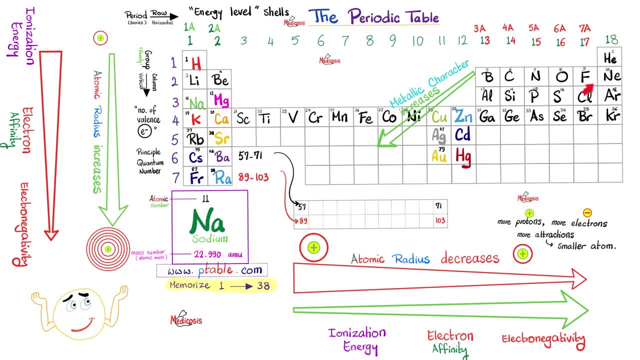 Fluorine, which means as you go to the right and upwards, electronegativity goes up. Metallic character is the opposite. As you go down and to the left, metallic character increases. That's it. It's easy peasy. 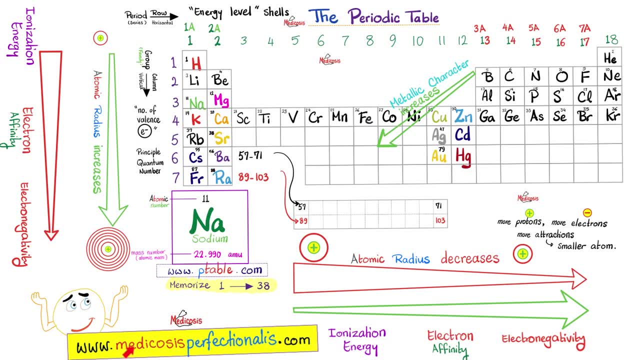 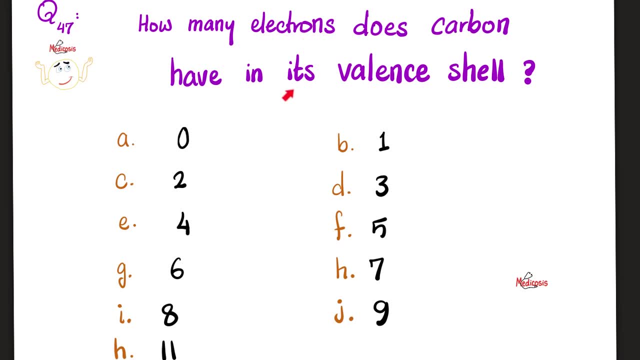 You can download my handwritten notes on my website, medicosisperfectionaliscom. Let's answer the question of the previous video. How many electrons does carbon have in its valence shell? I'm talking, of course, about a neutral atom. 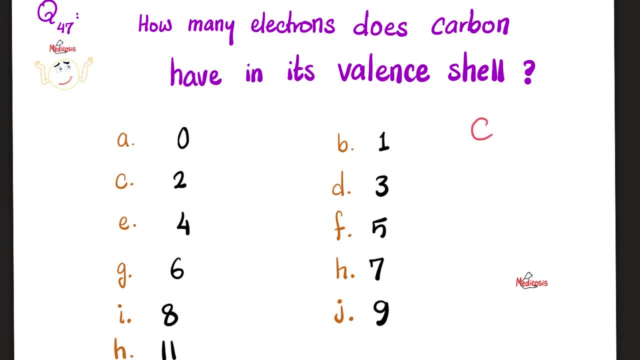 Please pause and try to answer this yourself. Okay, here is carbon. What's the atomic number of carbon? Six, Which means how many electrons does carbon have in total? Answer: six. Configuration based on shells, Not subshells, just shells. 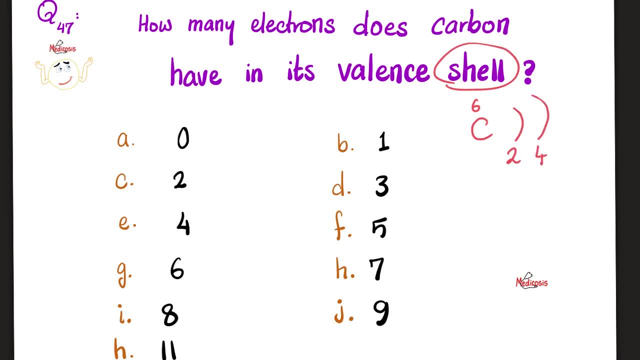 Two. Okay, how many are left? Four, So that the total is six. So the first shell has two, and then the outer shell, or the valence shell, has four. So the answer here is four If you have one or two or three electron in the outermost shell. 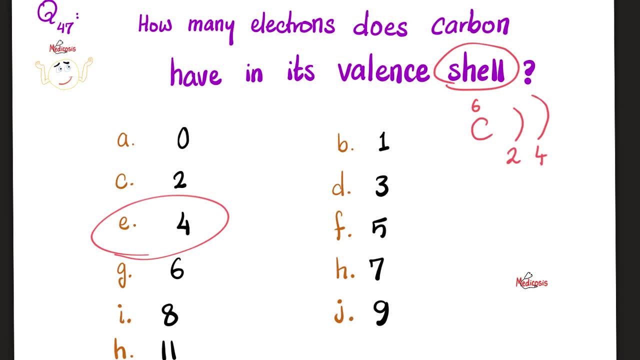 you tend to lose them to become a positive ion. But if you have five, six or seven electron on the outermost shell, you will tend to gain more electrons to become a negative ion. But what if you're stuck in the middle? 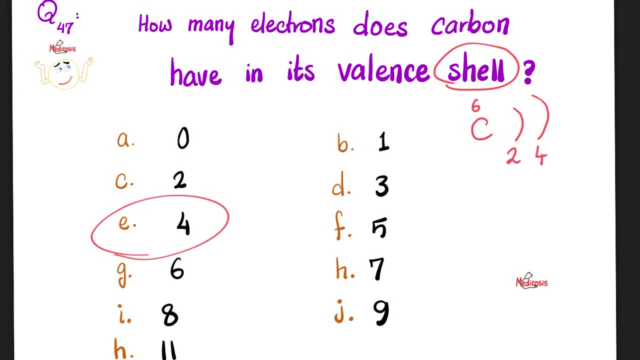 What if you have four electron in the outermost shell? Then you will neither lose nor gain. Instead, you will share electrons, ie covalent bond, And you will see carbon with four bonds with hydrogen, so that we are sharing four electrons. 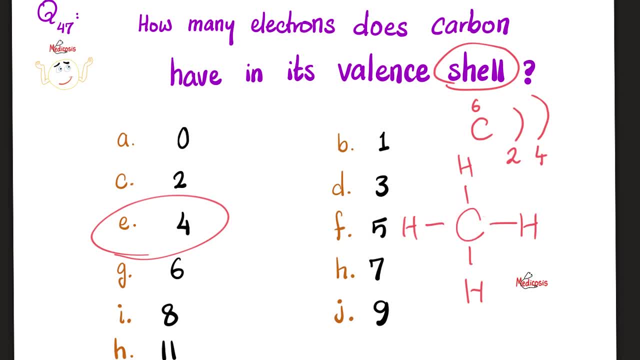 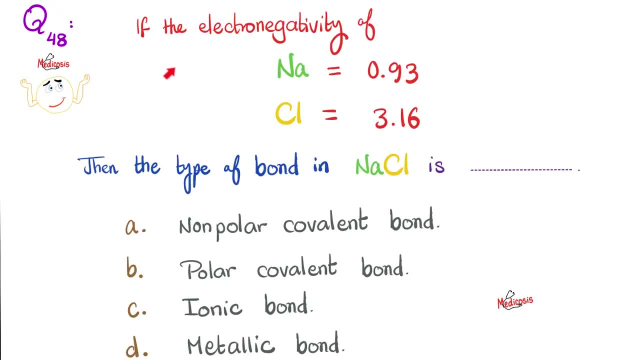 So now carbon has achieved the octet rule. And what's that? Hydrogen, Hydrocarbon, And you will see this all over organic chemistry. Question of the day If electronegativity of sodium is 0.93 and electronegativity of chlorine is 3.16,.